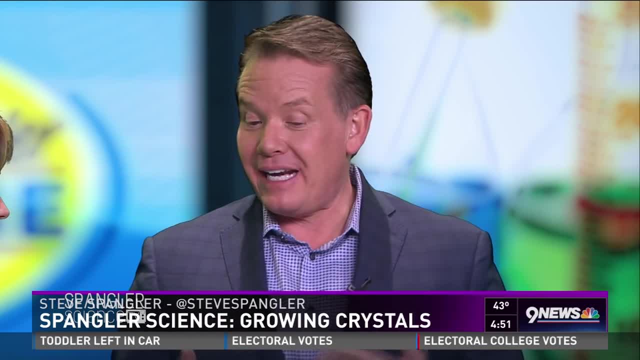 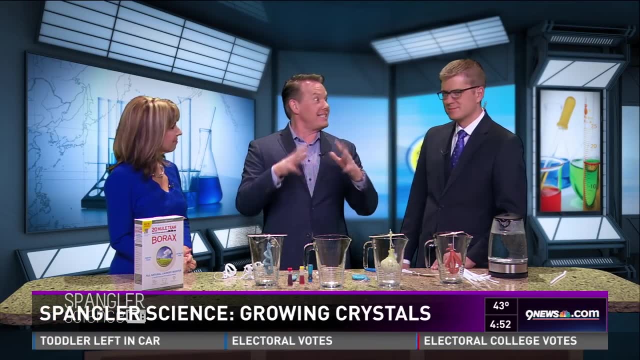 a cart and I put the stuff on the cart and I moved from room to room to room. I got a chance to see 27 teachers teach at their best, because that's what teachers do. Sometimes we put them in the room and shut the door and never get to see them. just be excellent. 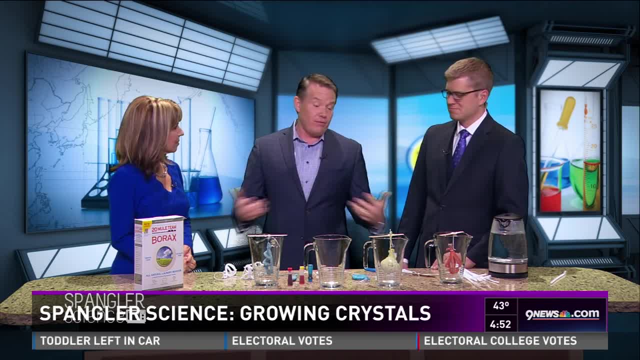 And as a brand new teacher, I got to see 27 amazing teachers. Unfortunately it didn't rub off on me, but I got to see it Very funny. So that's kind of how it works, But you teach us science every day. 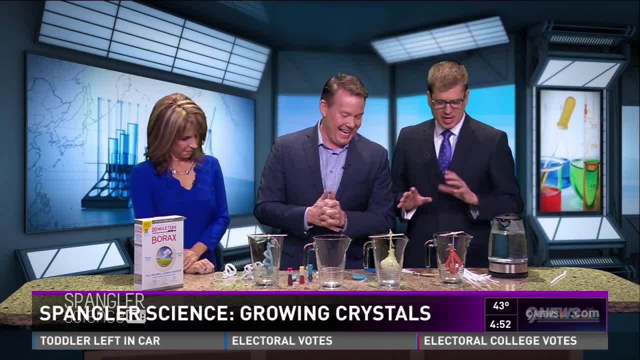 Very cool. I feel lucky. I feel like there's a minimal probability of you lighting me on fire today. Well, look at this, and your suit's not going to get a hold of me, Megan's scalding me. You're going to be fine that way. Hey, I thought it would be kind of funny. You know so much. 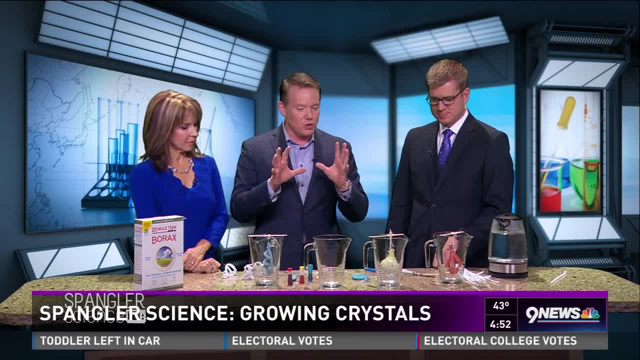 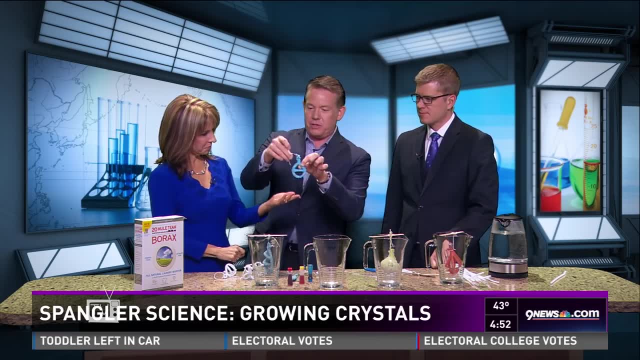 of the time we're blowing things up and fire and whatever else. This is just one of those really cool things that happens. It takes a couple of hours. You wake up in the morning and you go: my gosh, look at the Christmas tree ornament that we produced. Look at that. 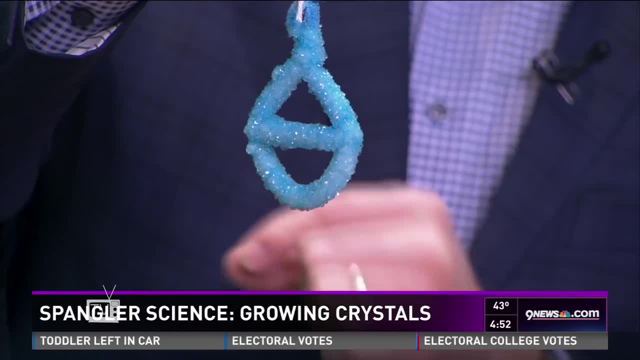 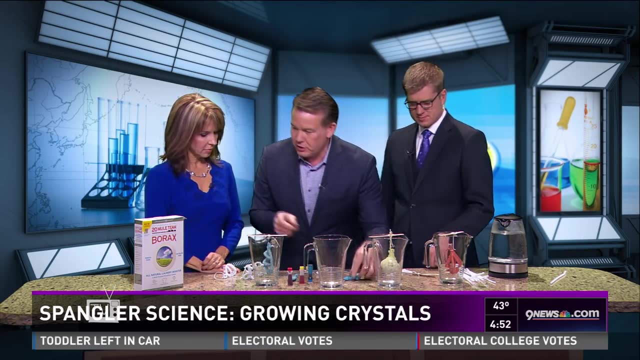 Isn't that just absolutely gorgeous- All sparkly and wintry. All sparkly and wintry and pretty, Really really easy, and it teaches you a quick little lesson in crystals as well. Okay, So here's what we started with. You kind of start the solution, So I'm going to use some 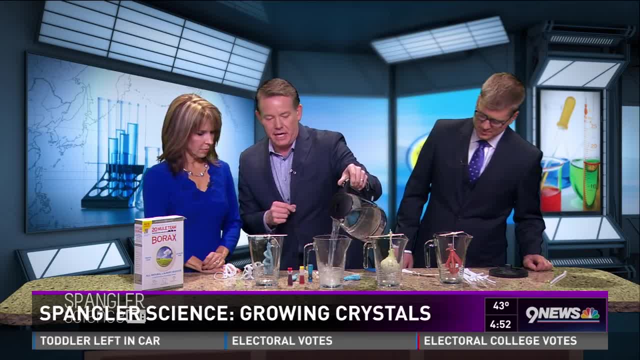 of the hot water. if you don't mind, Go for it. The hot water goes in here. You can make it any container you want. I wanted it just a little bit bigger so that the crystals won't touch the sides, Okay. 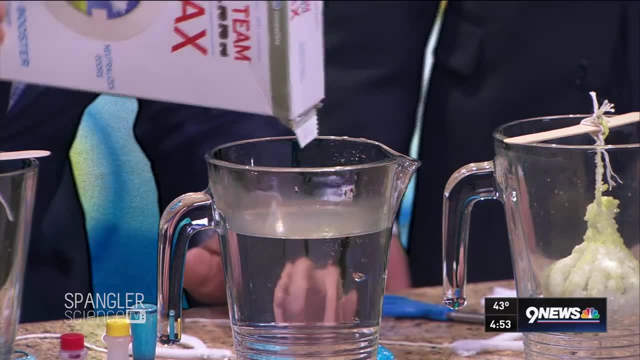 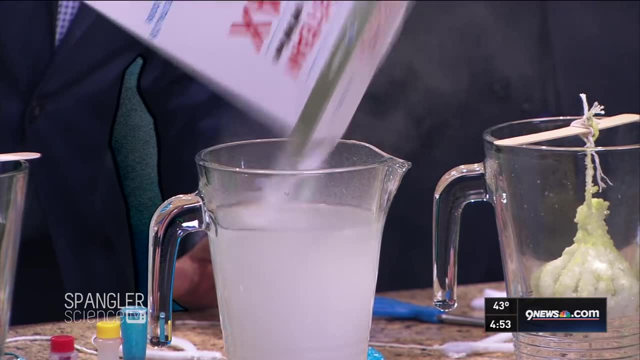 All right, And then we're using borax, so excuse the reach. Borax, Borax, So you mule team borax. Science teachers seem to use a tremendous amount of borax. We make slime with it and goo and all those other things You're going to want to make. 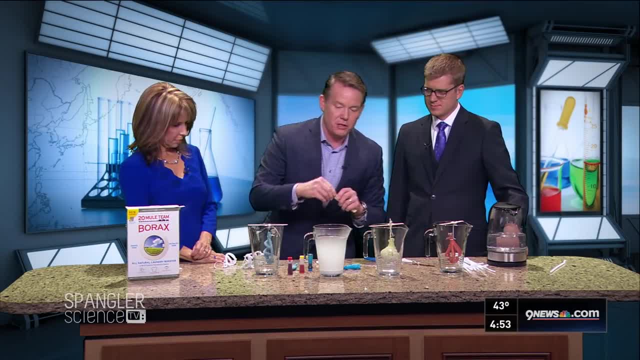 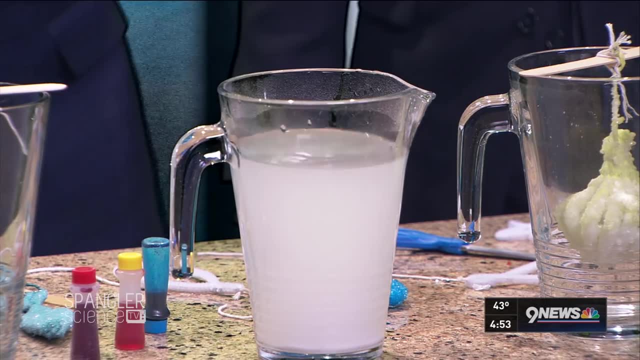 a saturated solution. So this is not going to be. we'd spend some more time with it, but you're going to stir it around, let it dissolve. The reason we use the warm water is we want to open up the space between those molecules a little bit more and stick more. 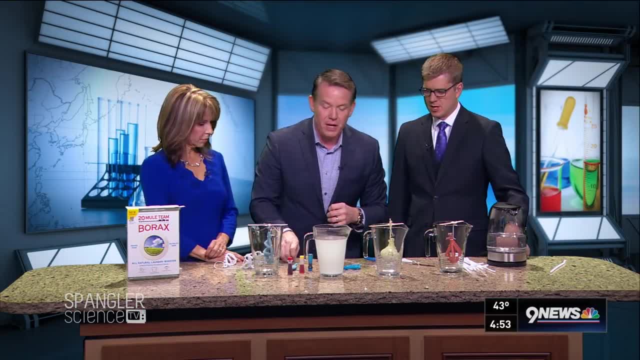 in. So when it starts to cool it'll crystallize and come out a solution Harden around whatever you stick in there. So here we go, We're going to get that going in there, and then you can add whatever food coloring you want. 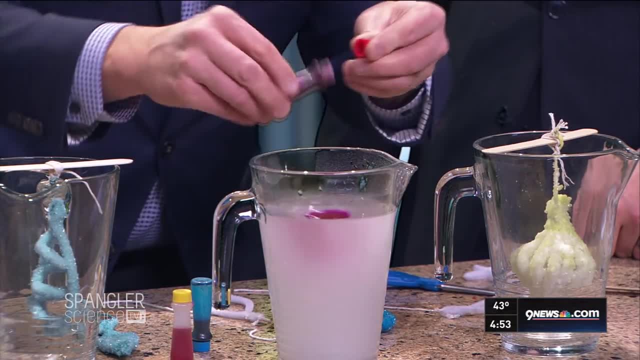 Color it up. Let's just say that we're going to color it up like this, And so now it's time to be able to make the next part, and that uses those pipe cleaners that are there. What do they call them now? Chanel sticks or something like that. 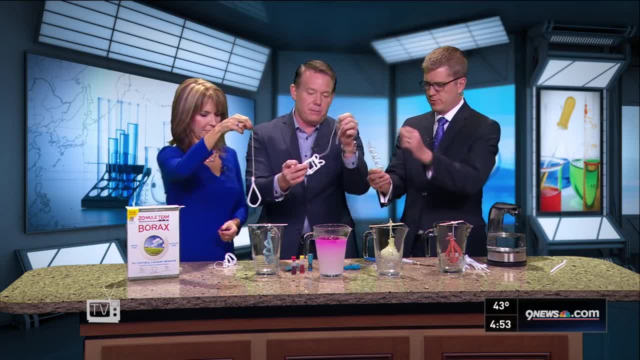 I know Pipe cleaner people Kind of do whatever you want here. So look at what you can do, but you can make some pretty cool things. Yours is very nice, very, very nice. So what you do now is that you take and you're going to wrap this around. 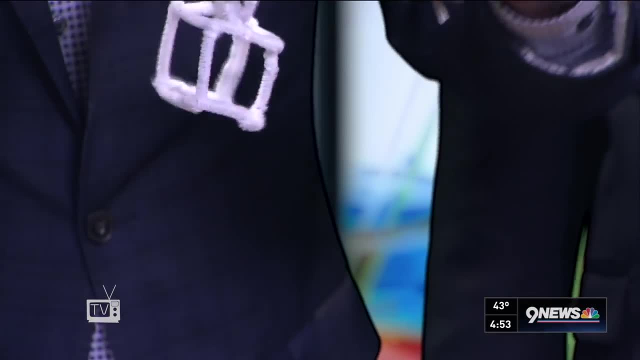 a popsicle stick like this. I have one done. You do have one done, Very, very nice, And I think you're just asking for extra credit. That's what you're doing. That's exactly right. You didn't know that about me. 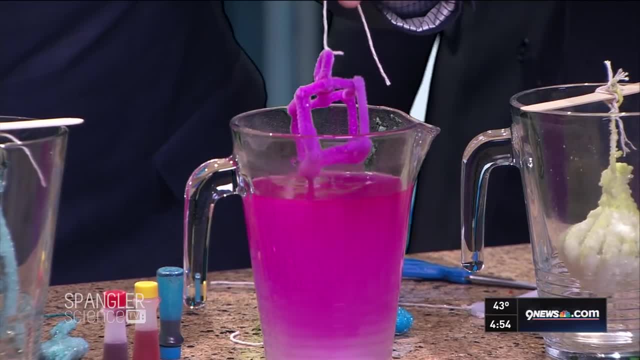 No, not at all Okay. And so now that goes down inside. Oh, it sits there. So you see this. So you stick it down inside. Oh, wow, Okay, the color goes on quick. That's just the color on quick. And now you let it sit there And as it cools, now the 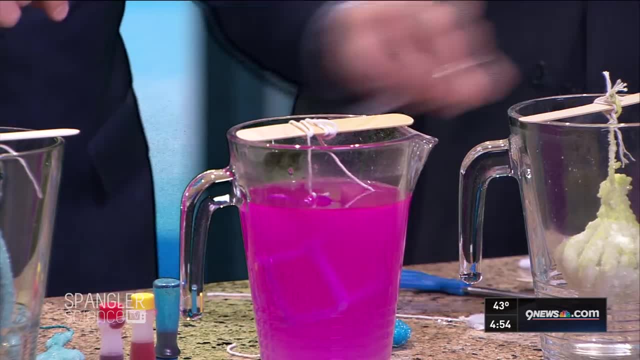 crystals start to crystallize And this watch what happens. Go ahead, pull that one out, Take a look at that one there. How long does that take? typically Maybe three, four hours. Okay, But overnight put it back in again. take a look at it back out again. You get some. 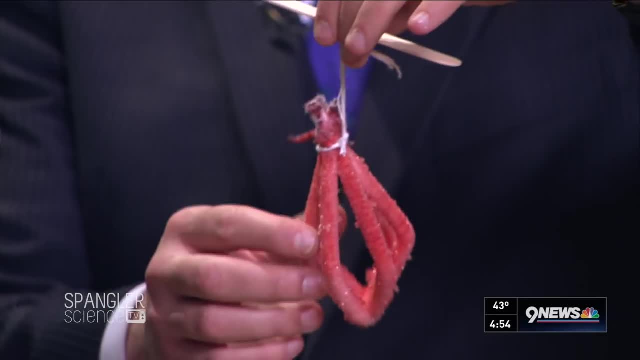 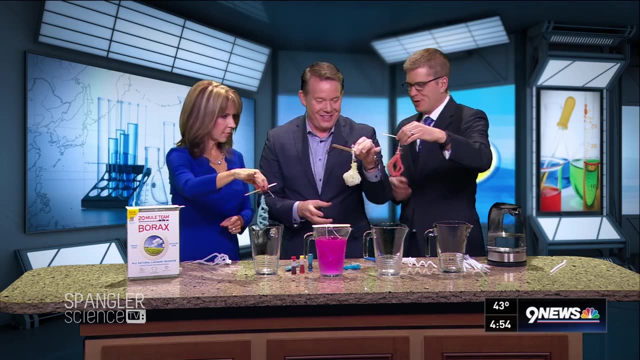 of these most beautiful crystals. So under a magnifying glass, of course they're gorgeous, but they catch the light And as they twist And actually it's not rubbing off like as much as You thought it was. Yeah, I would have. 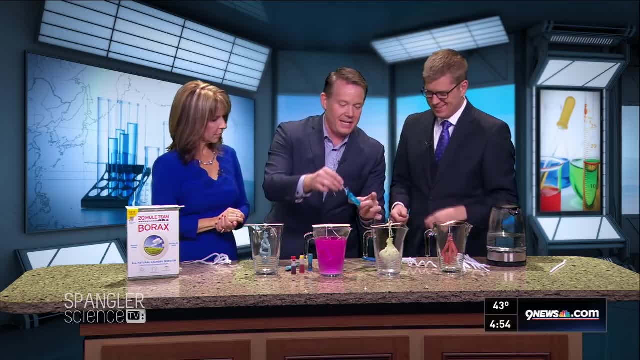 Yeah, I thought it was some of the actual, like store-bought ornaments I have. I was just waiting for you to say to me: is this dangerous? And I'd say no, the burning sensation will go away in a couple weeks. 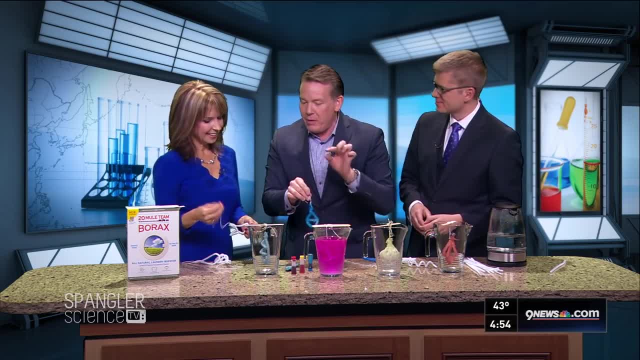 Oh good, So it'll be just fine. Fortunately It's fine. But isn't that beautiful? A great way to build the crystals and to kind of grow the crystals. You can do it last minute, throw it up on the tree, and easy to do. 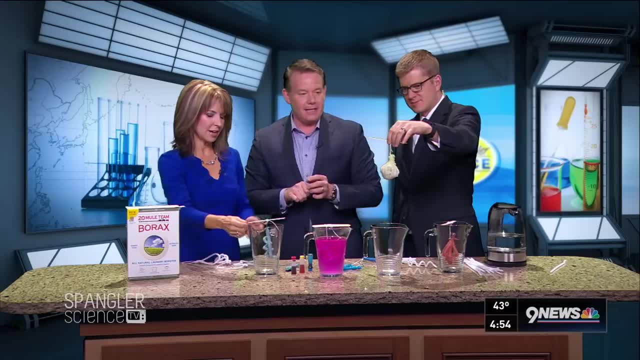 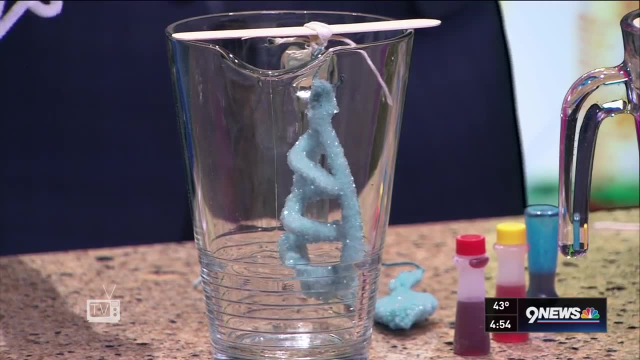 Honestly, these homemade ornaments mean the most Good memories. Kind of fun, isn't it? Yeah, And all for the boys. Hey, we put so much this year on the website And so a lot of parents are searching for Science Fair. They can go to the Nine News website and take a. 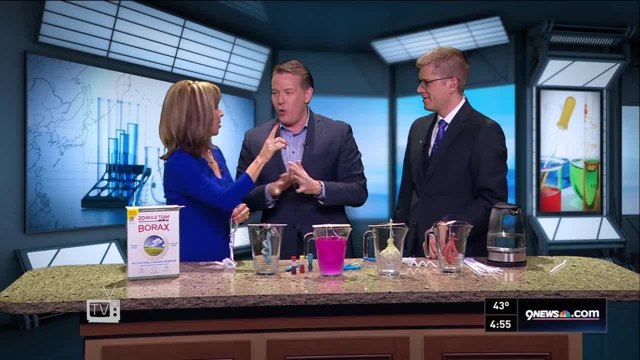 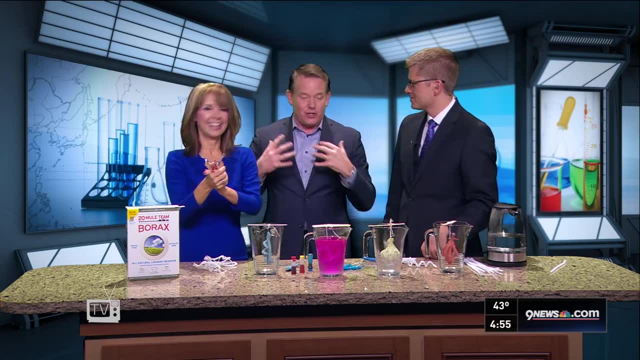 glance and see all those resources. So don't worry, Do yourself a favor. Don't worry Over winter break plan for Science Fair. Ladies and gentlemen, look right into my eyes. Do not make Science Fair one of those things where kids are crying right? We want this to be a great experience. 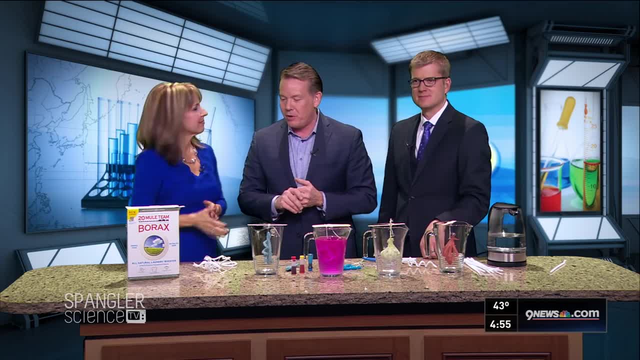 No, It's supposed to be fun. That's easy to do And we'll show you how to turn a regular experiment into something that they can really learn. My super basic question: if I don't put food coloring in, will it come out snow white?